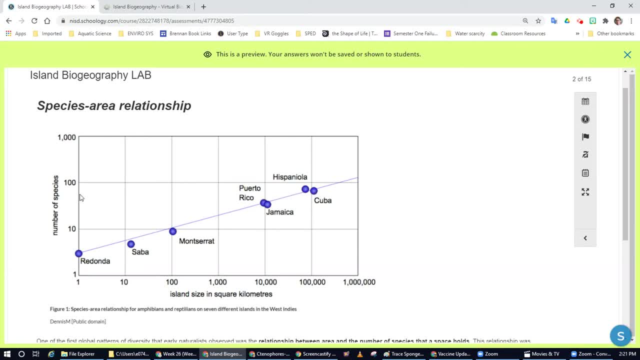 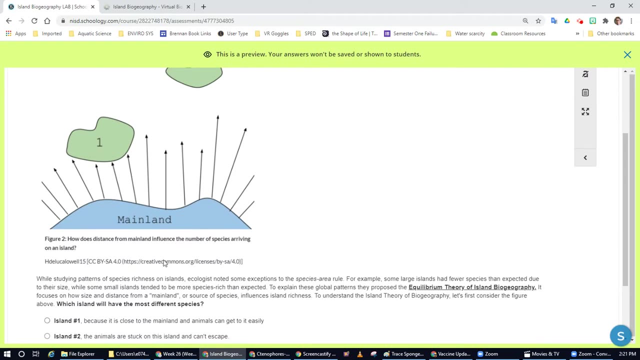 Cuba, And if you look at Cuba you can look over here to see what kind of biodiversity it has. So biodiversity would be: the more species you have, the more biodiverse. Okay, I'll leave that to you. to ask: Here's your mainland? and by mainland I mean the continent, the biggest land. 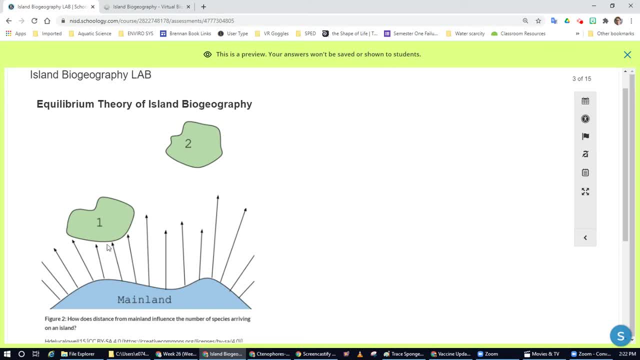 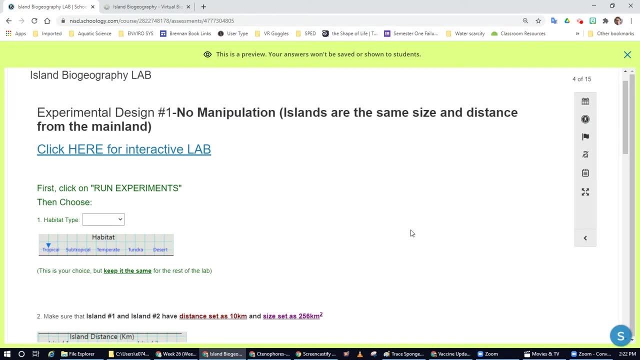 around And here you've got two islands: One is close and one is far away. just to walk you through that. Now here's the experiment. We're gonna do four different experimental designs. The first one is no manipulation at all. The islands are the. 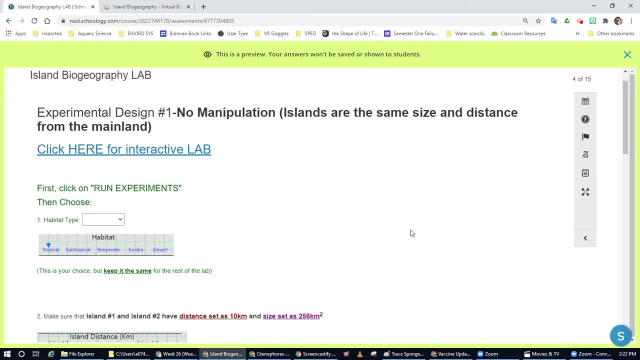 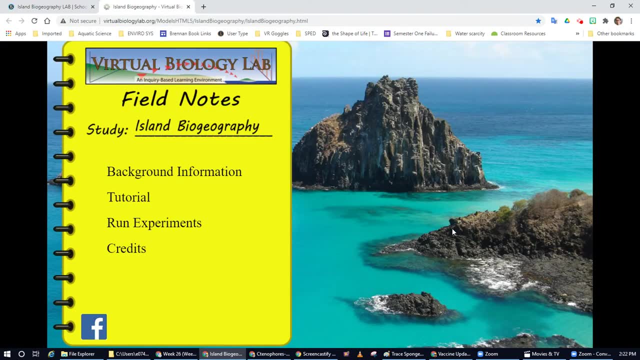 same size and the same distance from the mainland. So you're going to click here and this is going to take you to the interactive lab. The interactive lab: it's very beautiful. You can, if you wish, look through these different topics, but we're going to go. 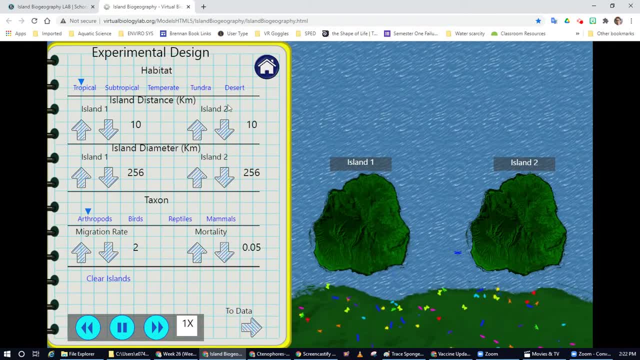 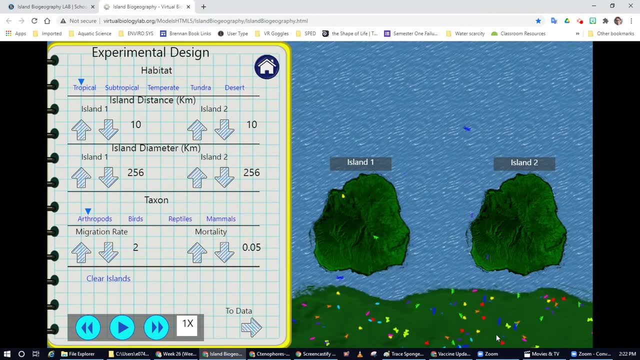 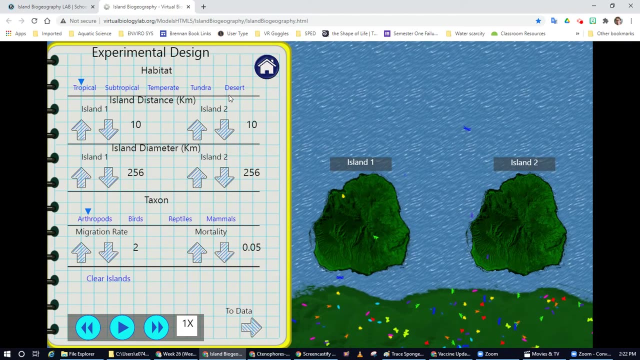 straight to run experiments. Now I've got an island here. I'll pause it. I've got two islands. Here's my mainland, the main big continent, and these are both islands that are 10 kilometers off the coast and they are both 256. 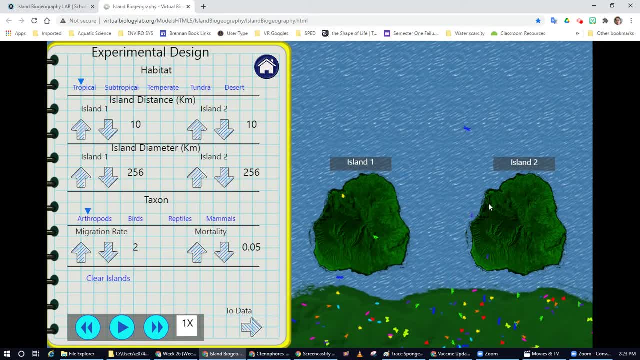 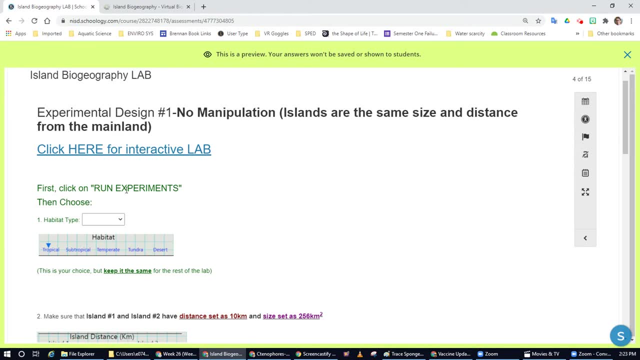 square kilometers. All right, so let's look at what we're supposed to do. So I'll go back to our Schoology. First we'll click run experiments, which we did, and then you're going to have to choose the habitat. 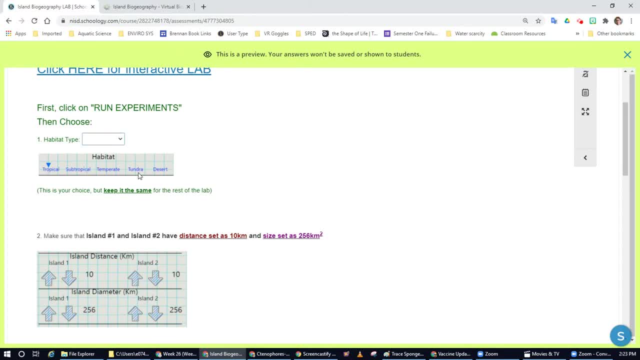 You have tropical, subtropical, temperate, tundra or desert. Now here's the important thing: You need to use the same one I'm going to show you. I'm just going to pick tropical, but it is up to you to pick. 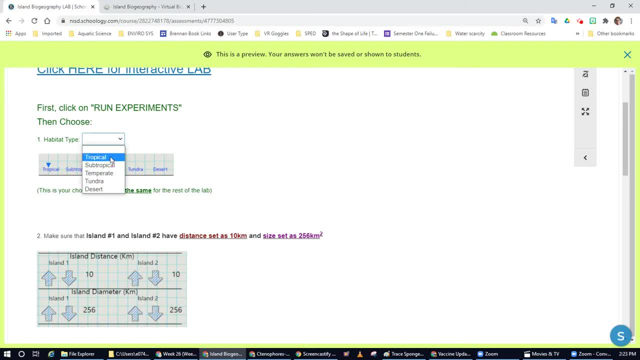 your own habitat type. So you'll come here, pick whichever habitat type you would like, and then you are going to keep that through all of the following experiments. All right, that's very important. Whatever you pick, that's what you're going to use for the whole lab. 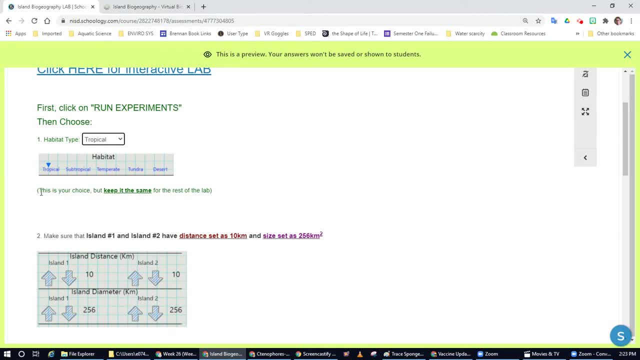 So we're going to use tropical. This is your choice. Keep it the same for the rest of the lab. All right, keep it the same. Island one and island two have the same distance and the same size. so 10 and 256.. It should look just like that. 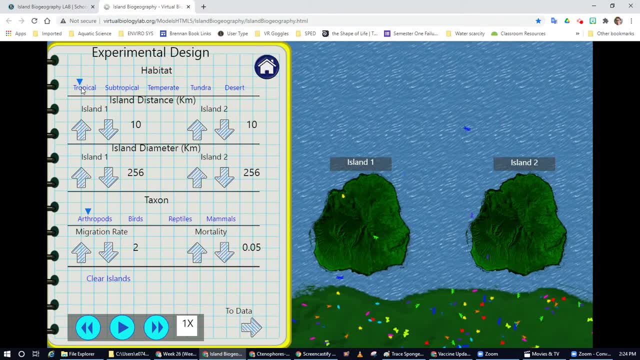 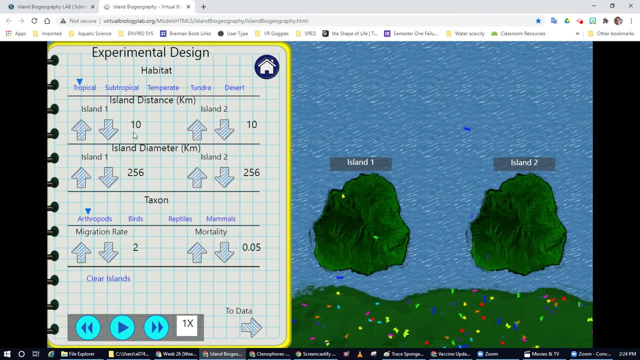 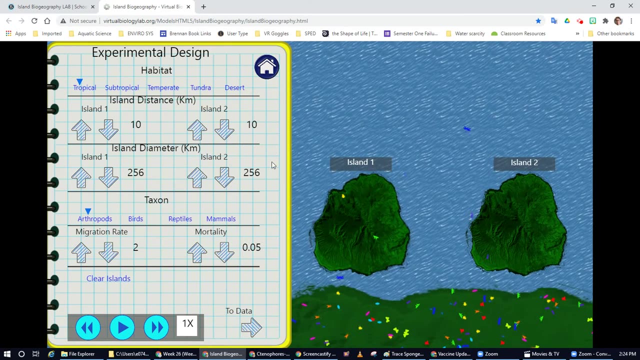 So we'll come over here. I'm going to pick tropical. You could pick anything you want, but I'm going to pick tropical for now. My island distance, as you can see, is 10 kilometers offshore. My island diameter, as you can see, 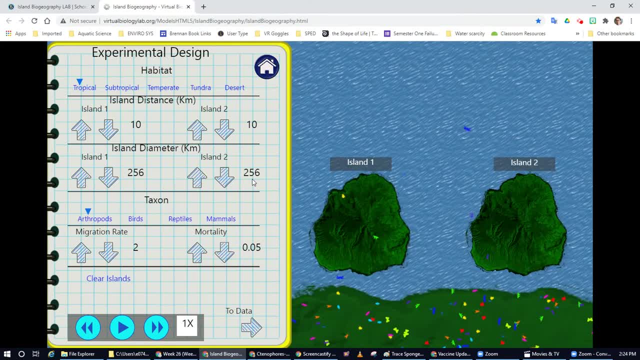 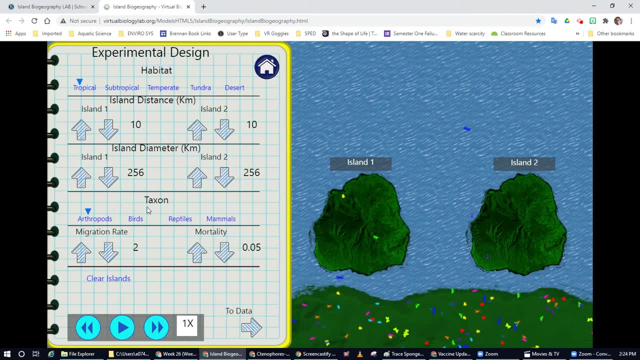 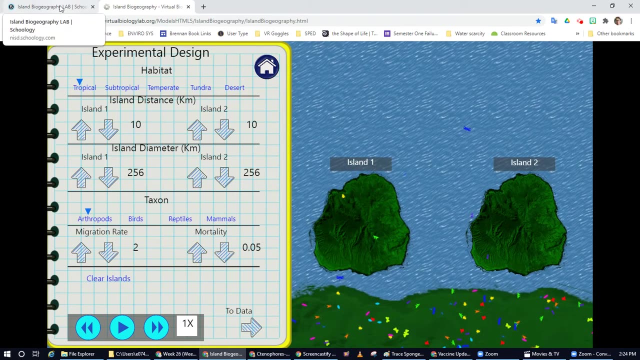 is they're both set at 256 for this first experiment, And then I get to choose the taxon- And taxon just means it's a fancy name. for what kind of animals are we looking at? You have your choice, and this is a choice that you will have to keep for. 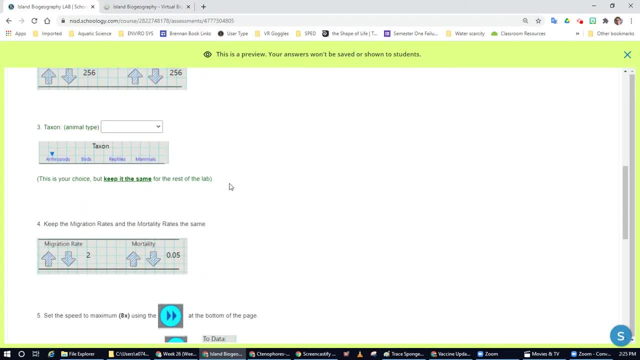 the rest of the lab. All right, your choice. Arthropods are bugs. You could pick birds, reptiles or mammals. I'm just going to go ahead with bugs Again, this is your choice. You need to keep it the same for the rest. 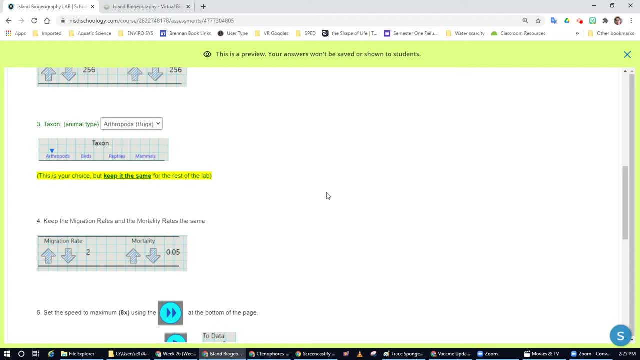 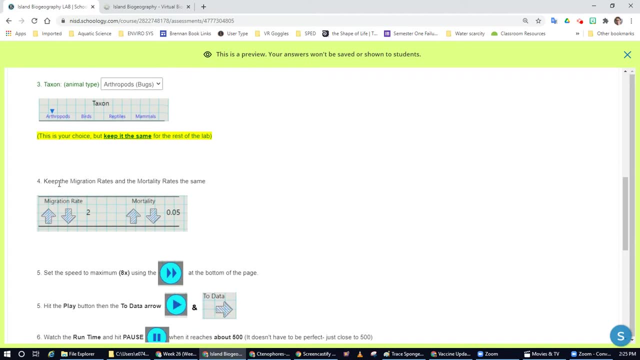 of the lab. Okay, whatever choice you make on number one, it doesn't have to be my choice, It's your choice. Whatever choice you make, that's what you keep. We are also going to keep the migration rates and the mortality. 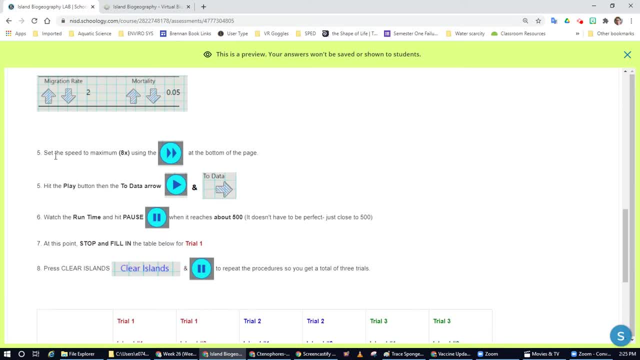 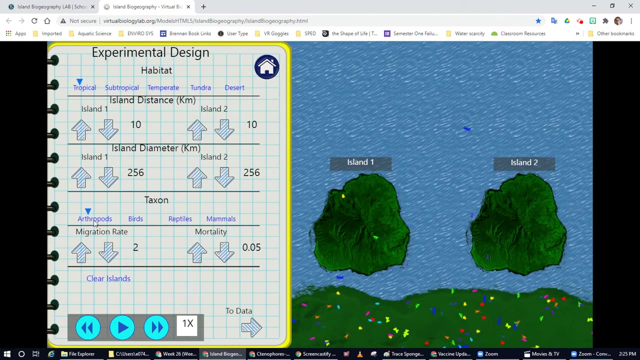 the death rates the same. Okay, you're going to set the speed to maximum eight times, so we don't have to sit around and wait forever. Then you're going to hit the play. So here we go. We have arthropods, which is what I chose. 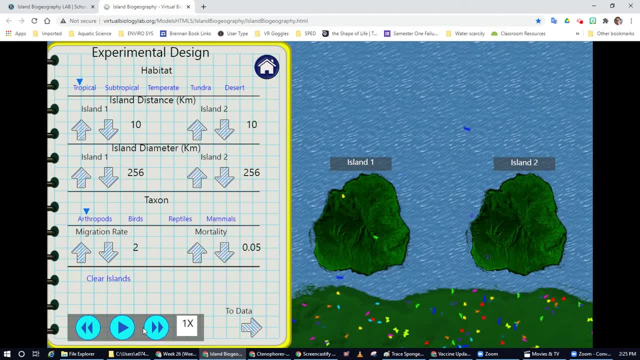 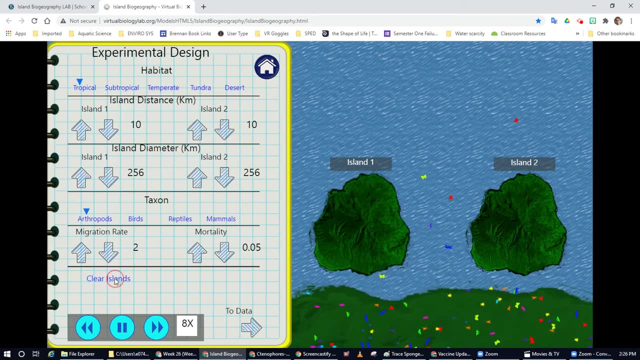 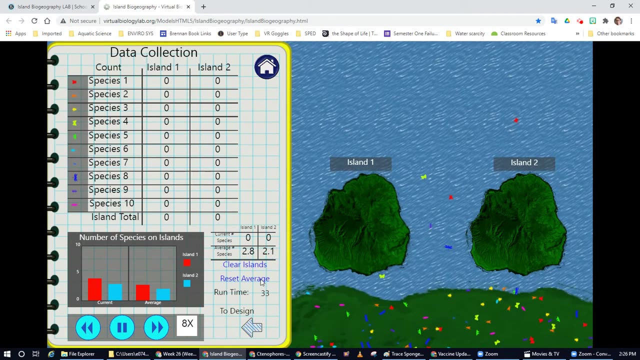 We're going to have the migration rate which is given, And I'm going to increase this to eight times. I can clear the islands, Clear the islands, so we get a nice early start And we'll come here and hit play. Now. we're going to do this for about 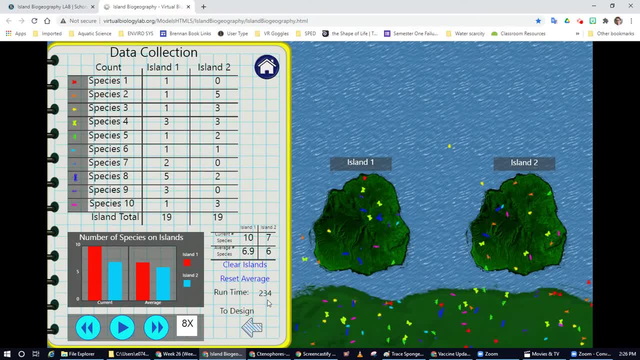 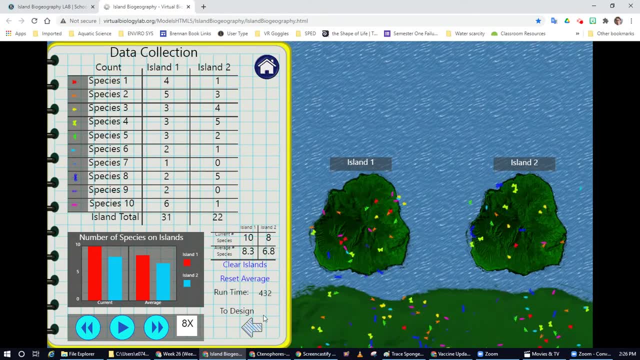 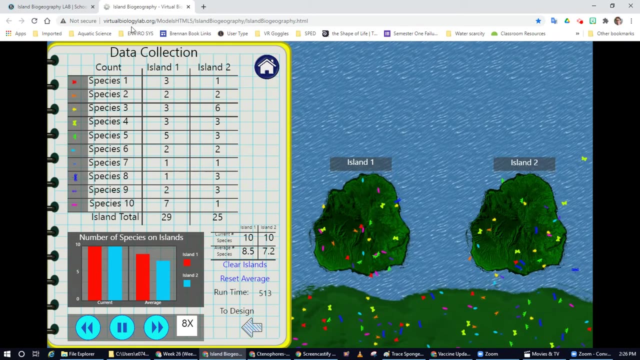 a hundred ticks of the run time. So here's your run time. You're going to get this to go to about 500.. Doesn't have to be perfect at all, So here we go. There's about 500.. Okay, now come back here. 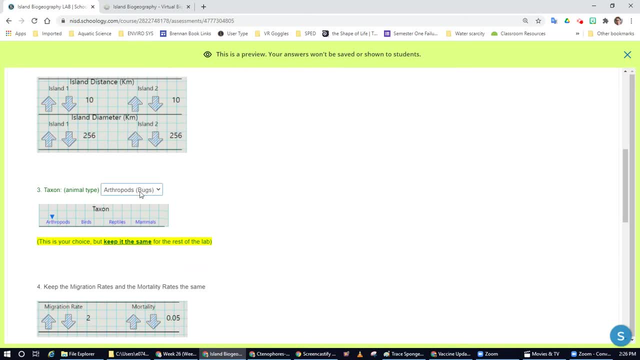 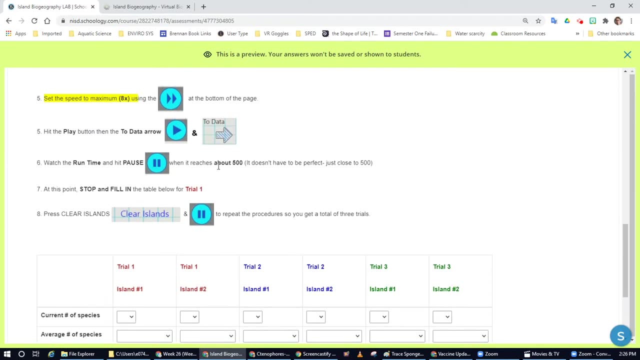 Double check: We've got tropical, We've got bugs. We've got the bugs. We're going to stop when it reaches about 500, just close to 500. At this point you're going to stop and fill in the table. 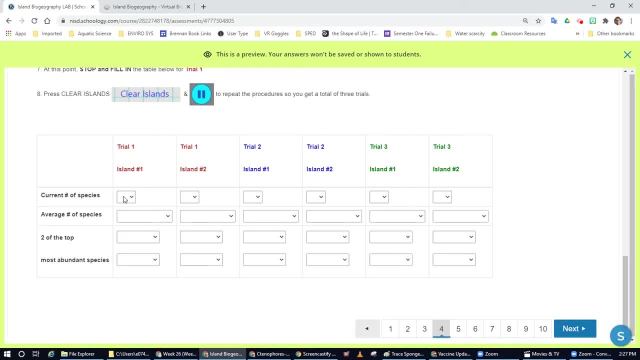 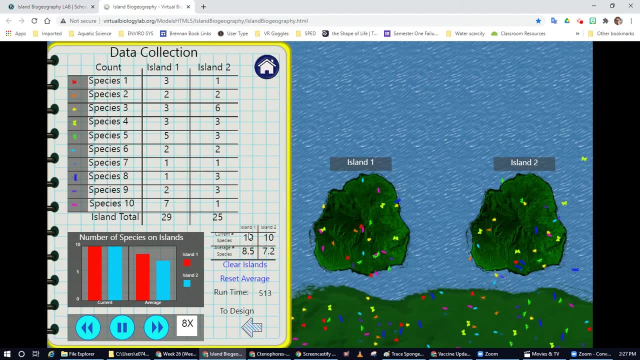 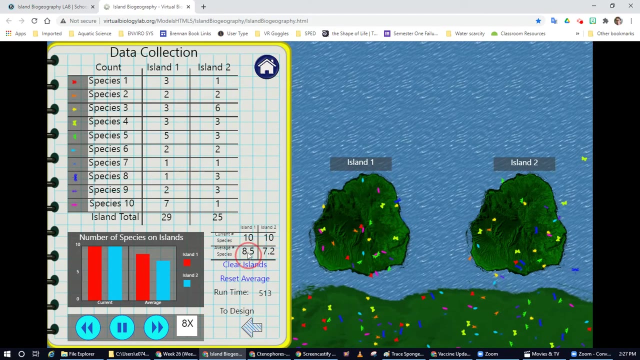 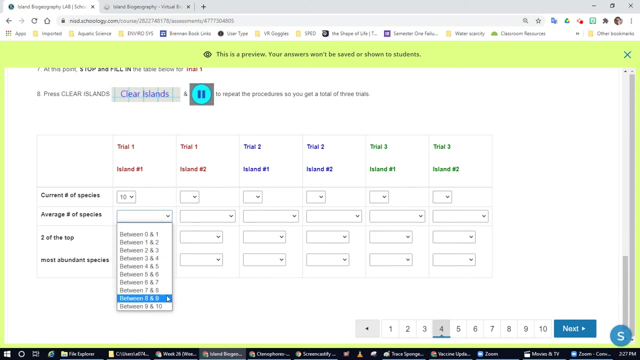 below for trial one. So trial one: current number of species. Current number of species is right here. 10. Idea number of species is eight point five. Now here I've got it between eight and nine. Eight point five is between: 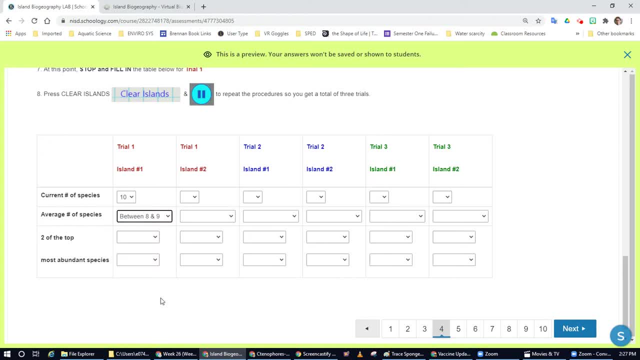 eight and nine. So I'll click on that. And again, I do know nine. if it's right at nine, you have a choice. See here: if it's right at eight, you have a choice. If it's right at nine, you have a choice. But you can see you'll get this. 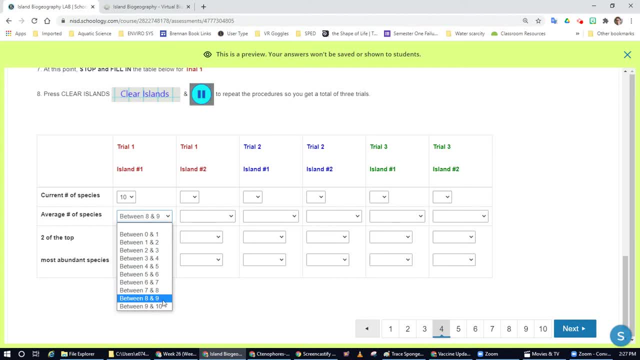 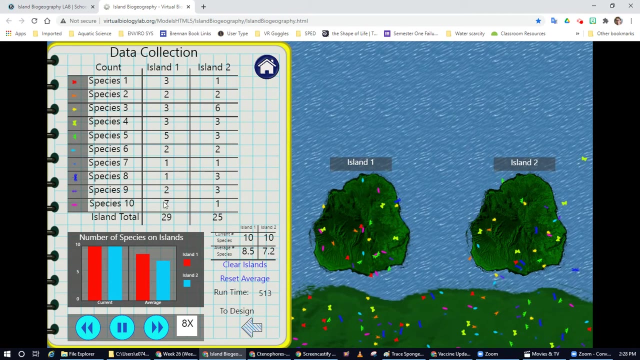 number, but use your best judgment on that, all right, And we're going to go. we're going to need two of the top most abundant species, So we're going to come here. I've got species 10,, which is at 7, and I've got species 5,, which is at 5.. 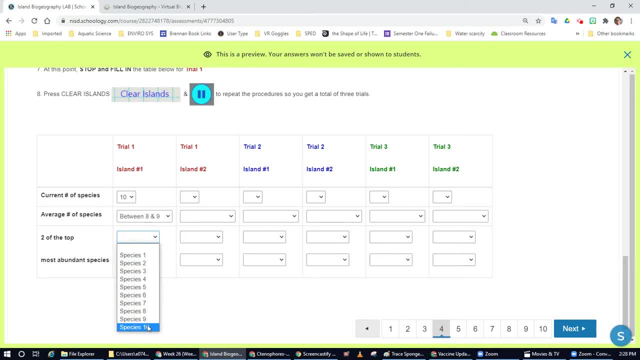 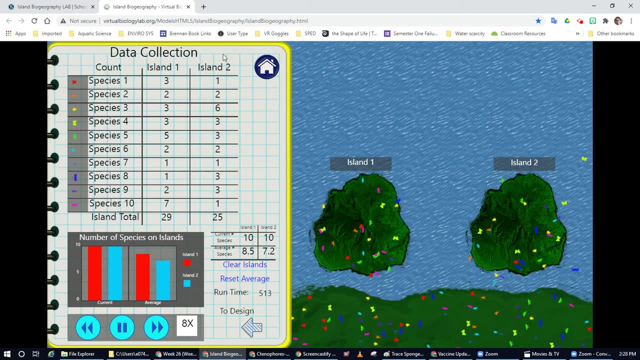 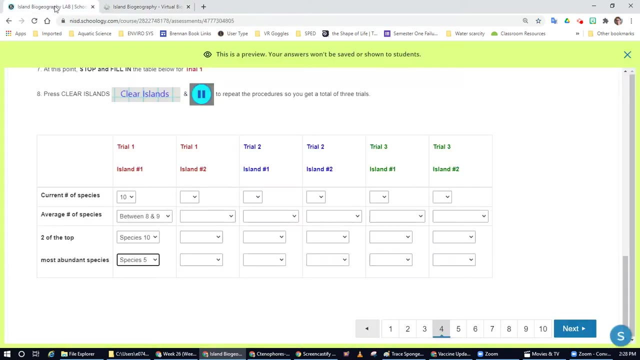 Okay, so 10 and 5, is that what I said? Yes, 10 and 5.. So now we're going to do the same thing for island 2.. If you look here, there's 10 species. 7.2 is the average 10 species. 7.2 is between 7 and 8.. 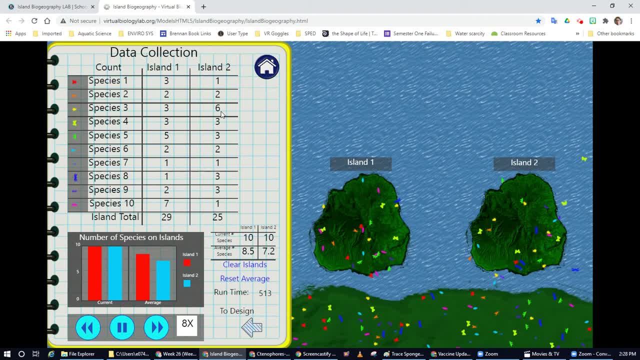 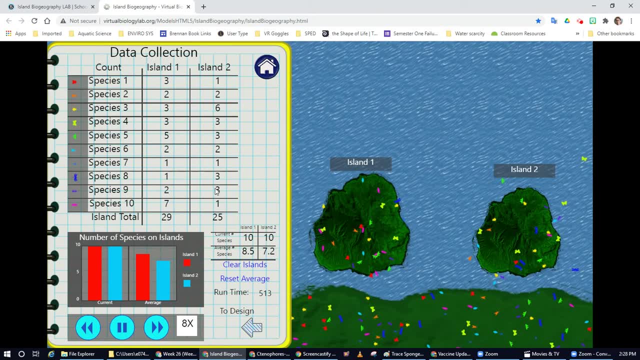 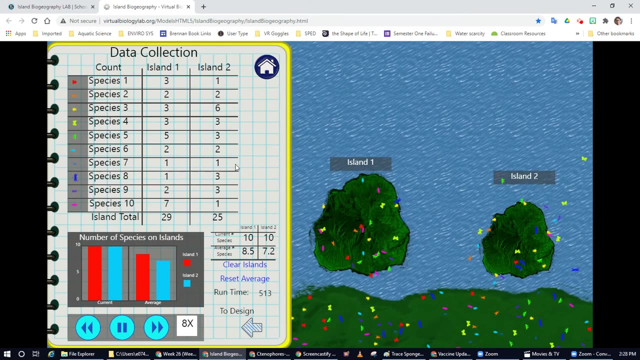 We're going to look at. we've got 6 species, Species 3, and then look at this: We have several. we have several different species that have 3.. So I'm just going to go with the top one right here: species 4,. all right, 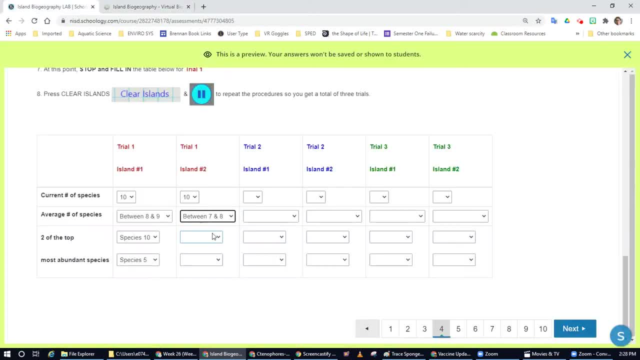 So we've got species 3 and species 4.. So I'll go: species 3 and species 4.. And now you're going to have to do the same. Do the same thing two more times, trial 2, and then trial 3.. 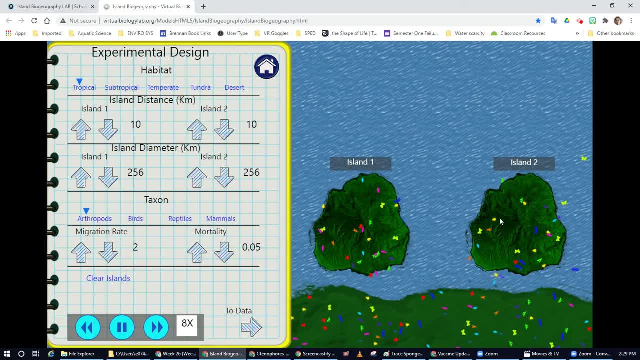 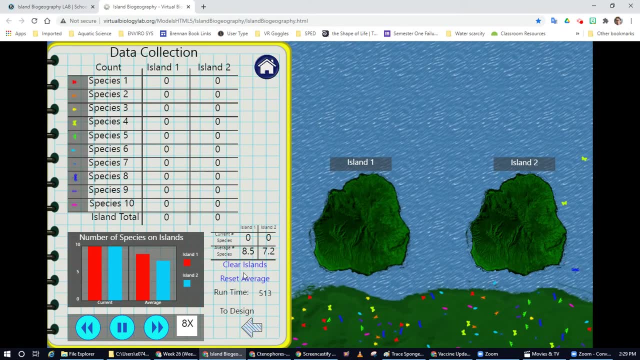 So we'll come over here. I don't know why I did that, but we've got. our islands are clear. We'll go over to the data Here. you can also clear islands and reset your average. We're all blanks here. 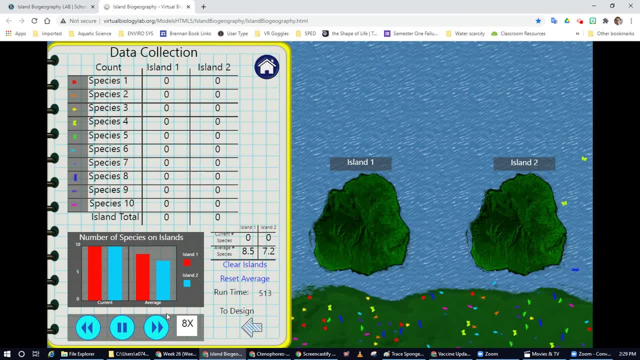 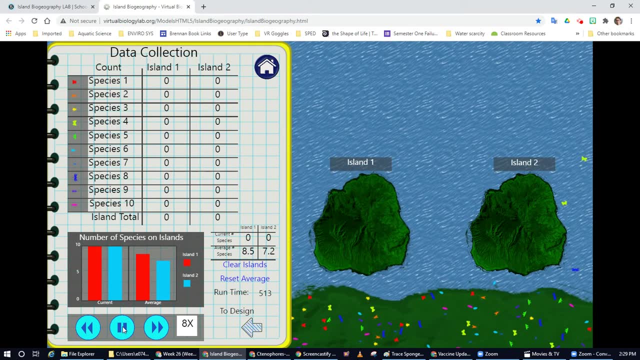 Don't worry about the leftover, It goes back to 0.. And now times 8, we're going to do it a second time. We're going to run this 3 times total, All right. So here the run time's going to be about 500. 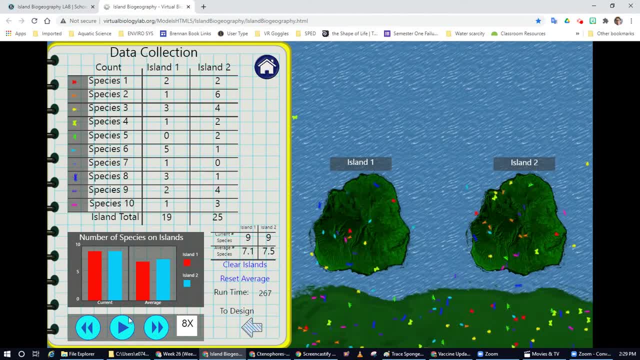 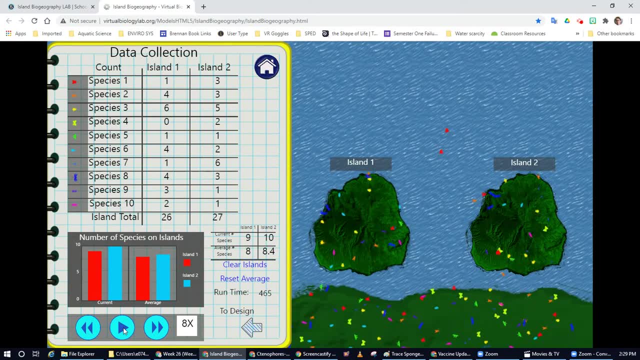 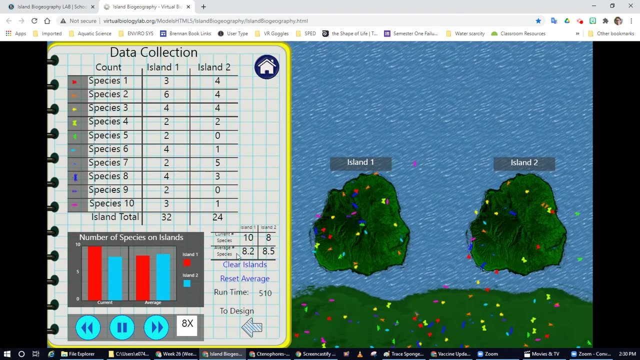 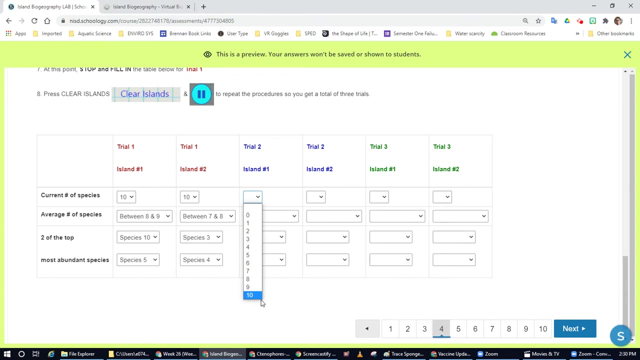 Doesn't have to be perfect. I'll come here. It goes pretty fast, especially since we've sped it up About 500, 510.. I got close. Now we're going to write these down. So, island 1. It's 10 and 8.2,. so we'll go here: 10 and 8.2.. 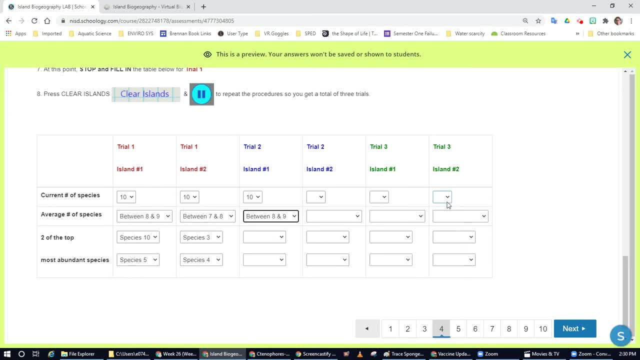 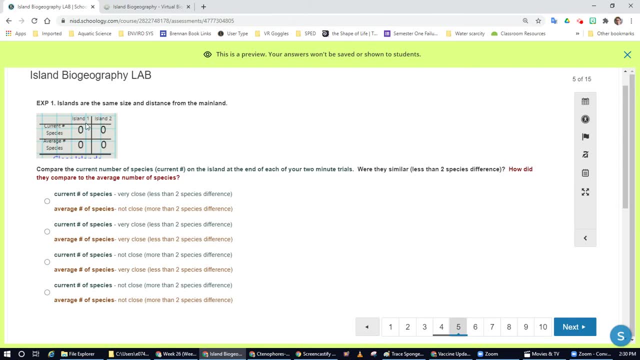 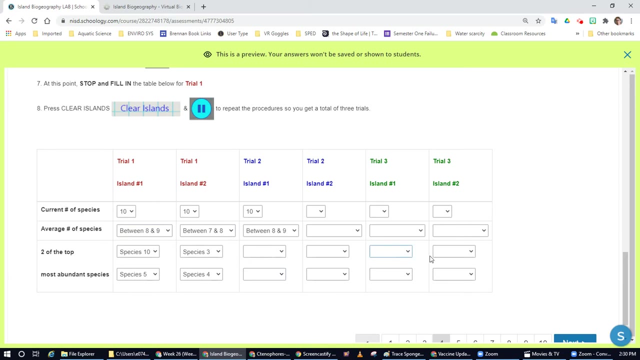 And you're just going to continue to do this. You're going to do it 3 times, All right, You're going to answer some questions by looking at the sum of what you get. looking at, oops, what you've put in here. which species you filled in? 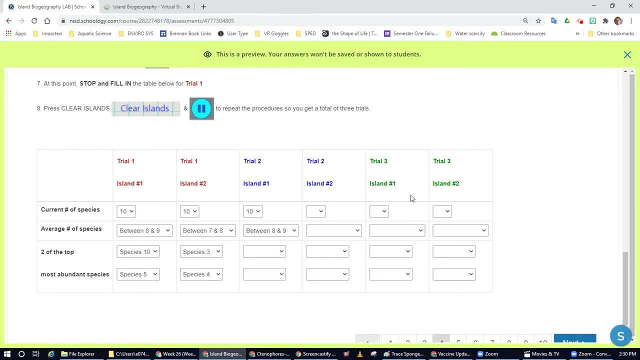 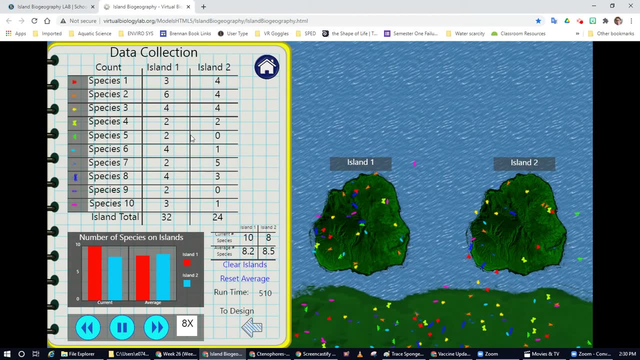 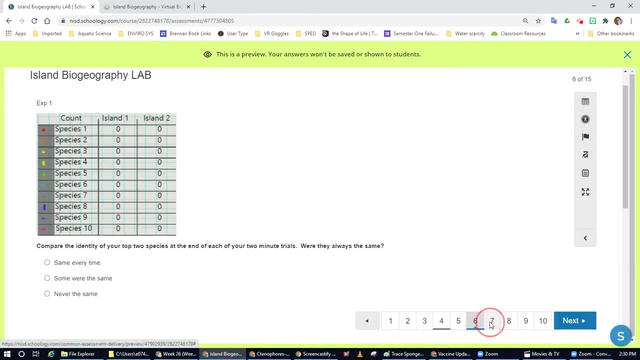 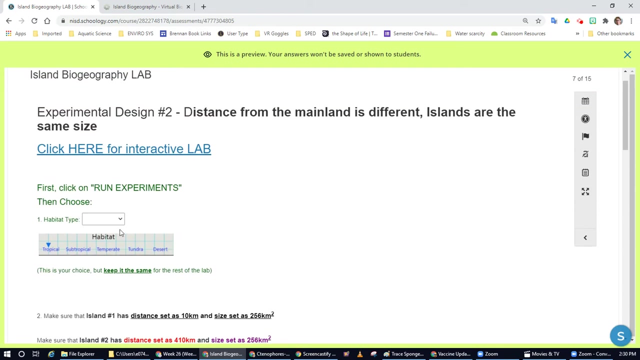 And remember, we're going to compare Island 1s and island 2s. Okay, None, Okay, Now for the next. we're going to have to change the distance from the mainland And it tells you again: you have to use the exact same habitat and the exact same animals that you used before. 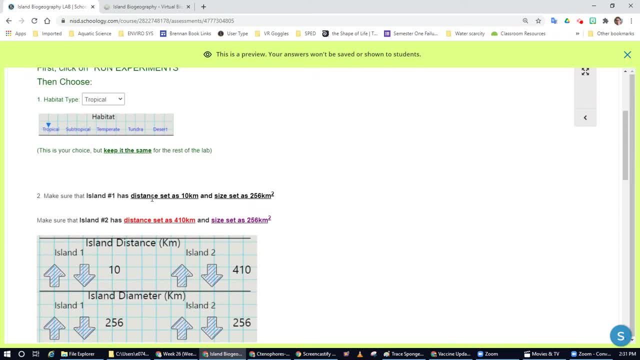